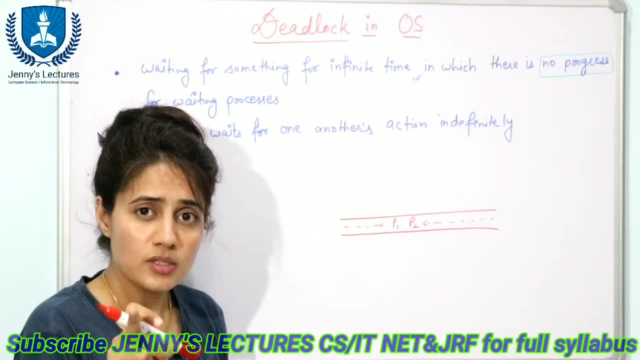 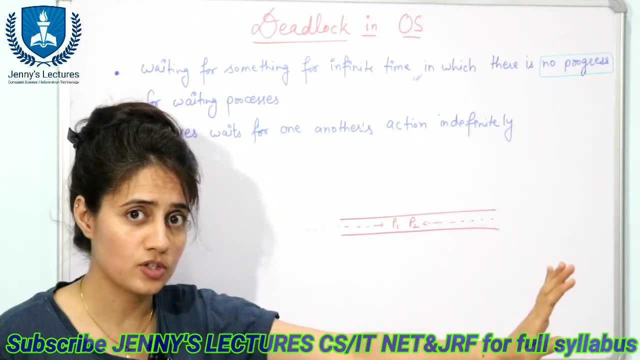 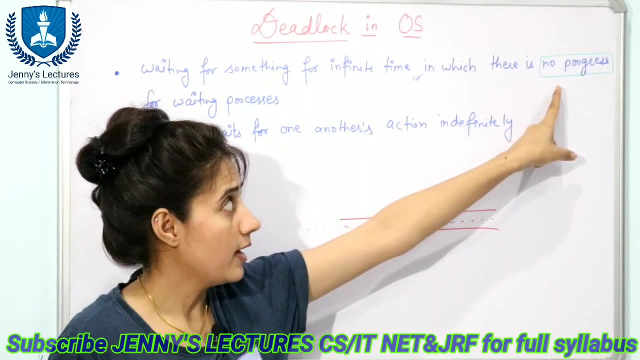 process. in starvation also we have discussed that waiting for infinite amount of time or you can say in indefinite blocking. but deadlock is different from starvation. in starvation we cannot say that there is no progress, but in deadlock we we say that there is no progress. if this word is there, no progress is there, then definitely there would be deadlock. this 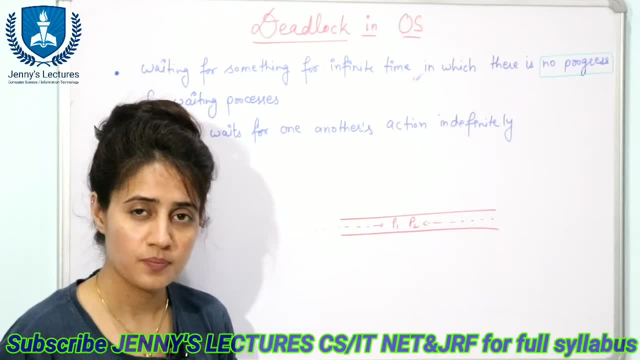 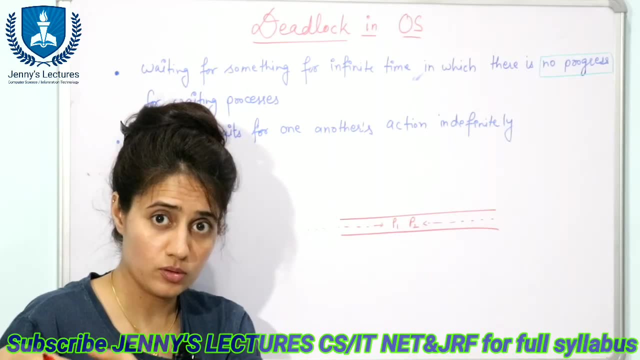 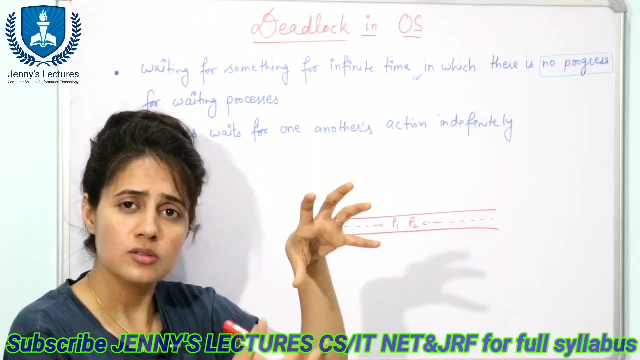 condition is: must means no progress. must in starvation, see, because of higher priority processes are coming, coming and coming low priority processes, will you know? wait, wait for the cpu. it's not getting the cpu, but here progress is there means cpu is running some processes. processes are coming and they are executing and they are going to terminate state. 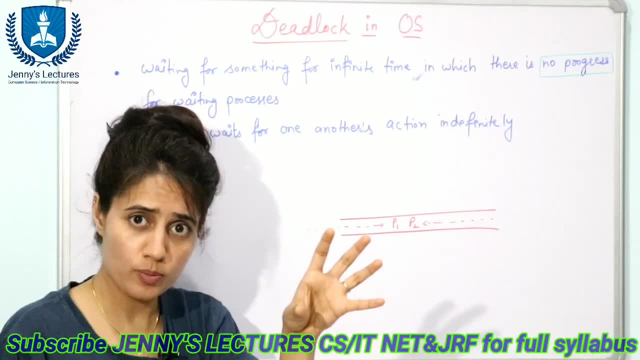 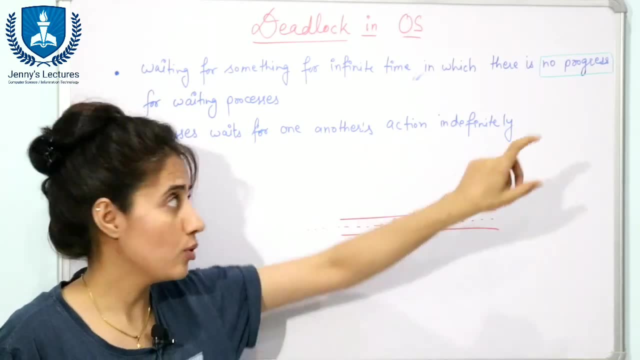 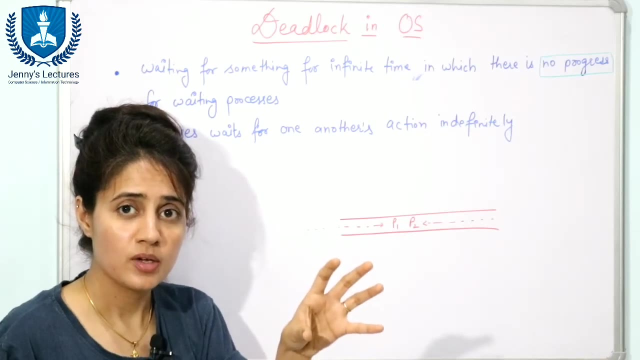 progress is there, but because of that priority case, low priority processes are not getting the cpu. fine, cpu is not blocked, but here here no progress would be there. then there would be deadlock. if cpu got blocked, cpu will not run any process. then we can say that the low priority 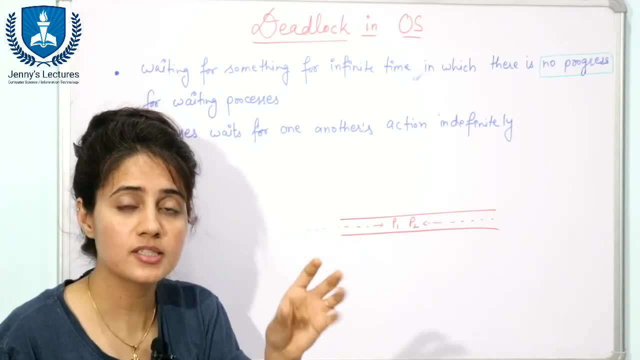 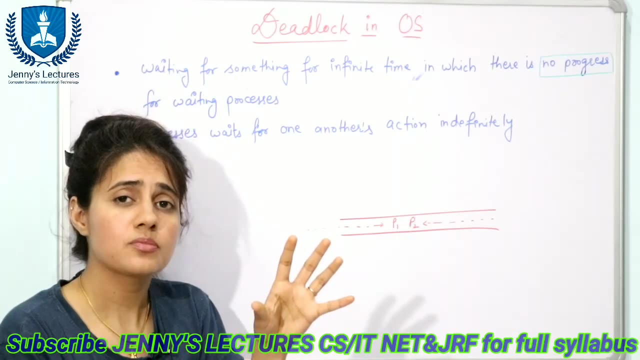 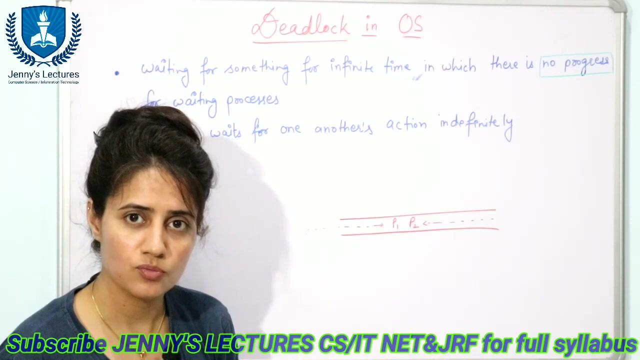 process will never get the cpu. but here, in this case, in case of starvation, maybe after 15 minutes, after one hour, after two hour or after three hour, that higher priority processes will not come and ultimately that low priority process will get the cpu because of the progress only, but if no, 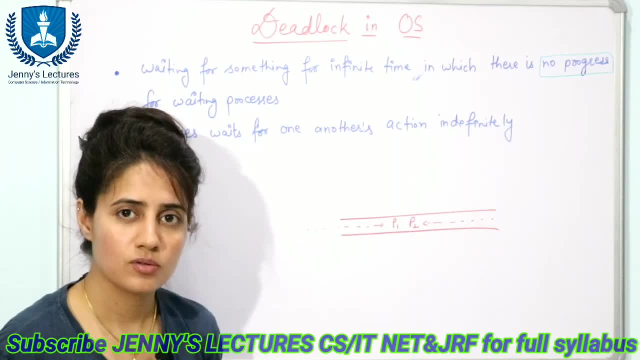 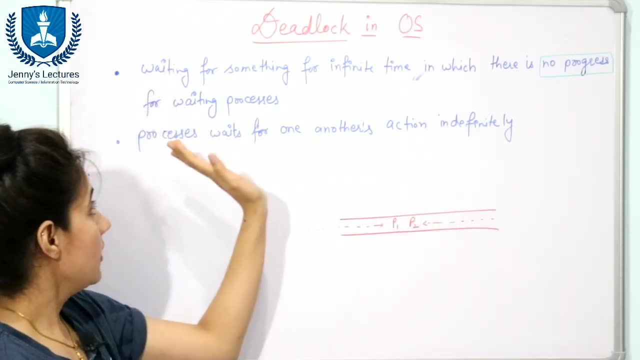 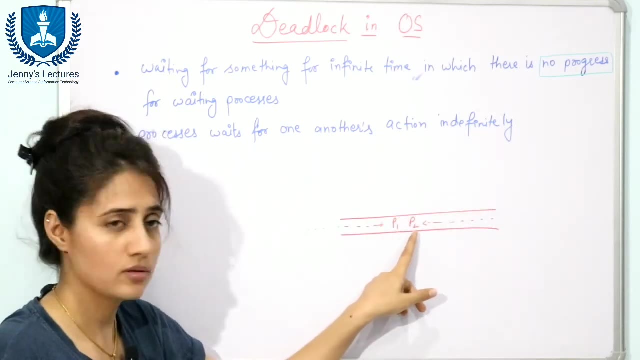 progress case is there, then definitely there would be deadlock. so this, this word is very important in deadlock: no progress. no progress means deadlock. or you can say: processes wait for one another's action indefinitely. here also you can say person: p1 is waiting for this p2's action and p2 is waiting for. 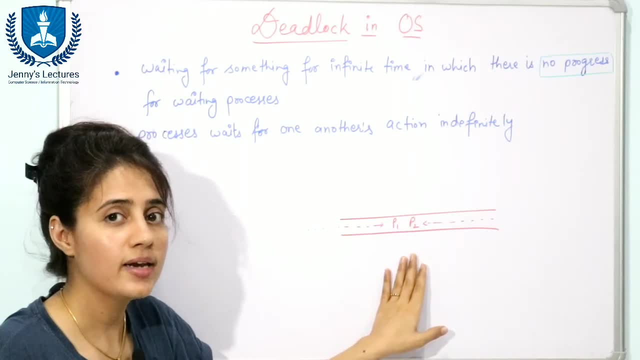 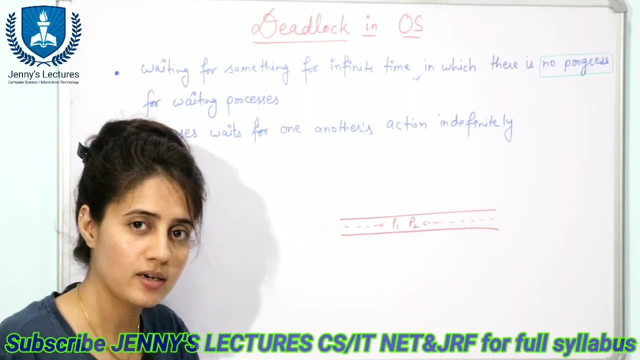 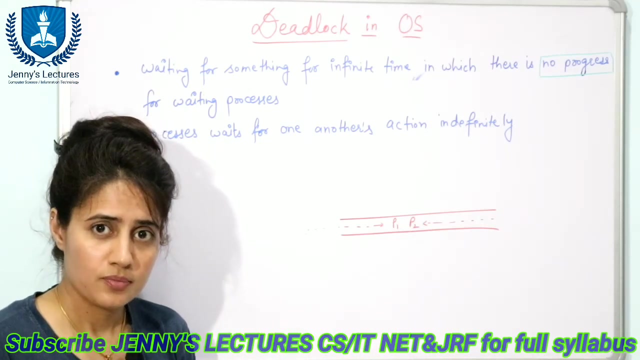 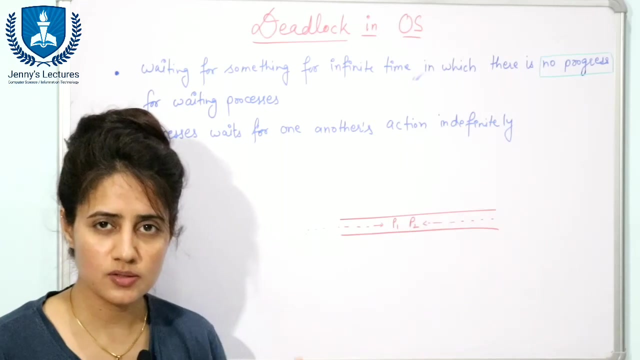 p1's action. but these action cannot occur. that is why they have to wait. the processes will have to wait indefinitely and that is the condition of deadlock. let us take one more example. suppose two children are there and they want to draw something and on one table one drawing book is there and one you can say a sketch pen, or you can say pencil. 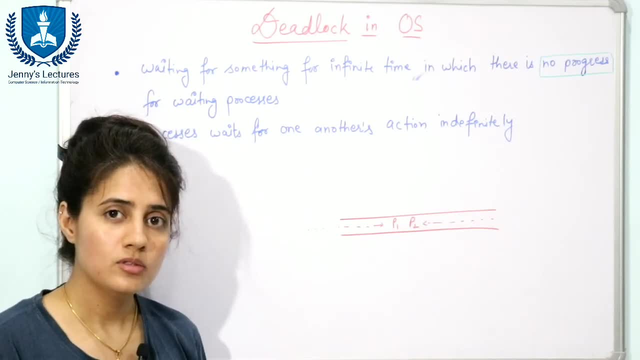 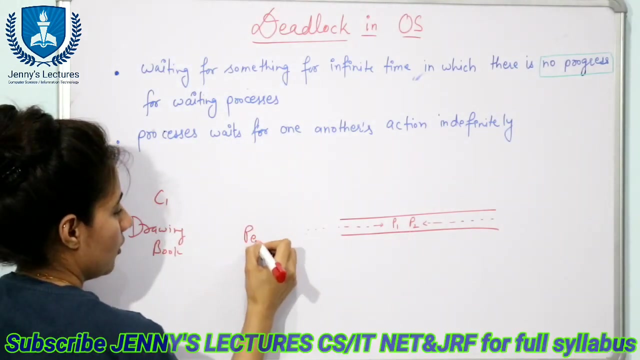 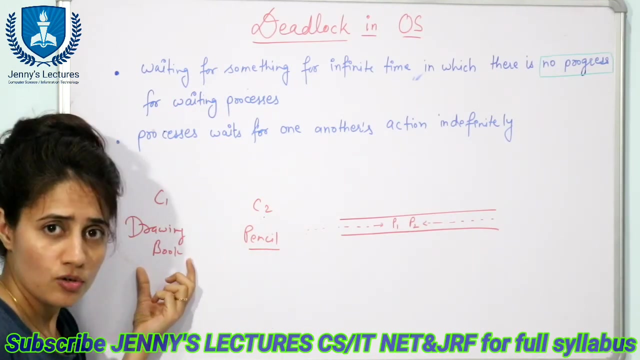 is there? fine, now they, they both the children, run to get the drawing book and pencil. now one child got this drawing book and one another child got the pencil. okay, fine, one child, suppose c1, and here we have pencil, and c2 got pencil. now neither c1 can. 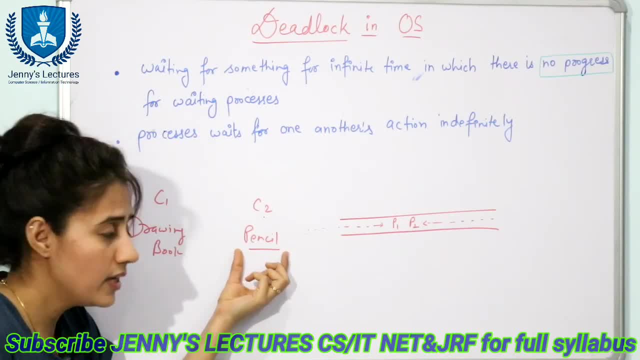 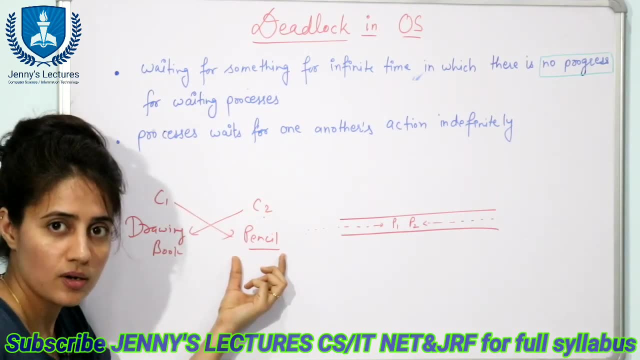 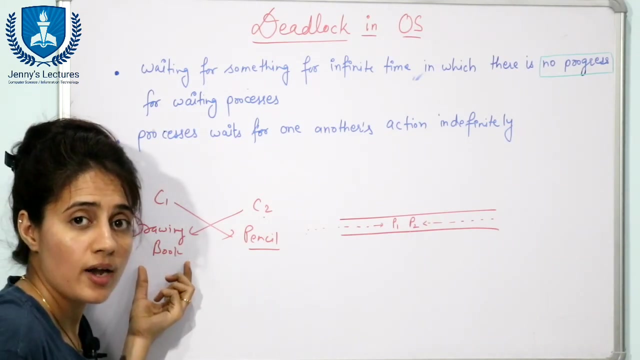 draw something, nor c2 can draw something. why so? because c2 only has pencil and c2 is waiting for this drawing book and c1 is waiting for this pencil and c1 has only drawing book. so both are waiting for resources which are held by some. 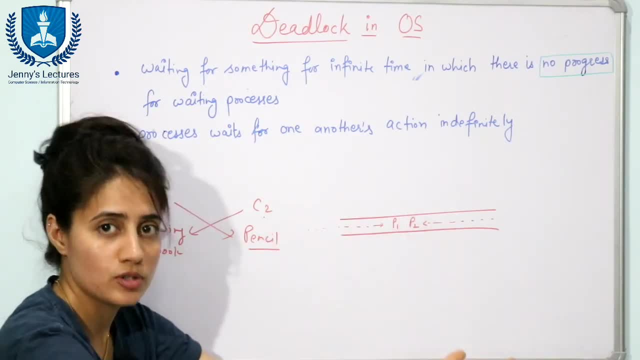 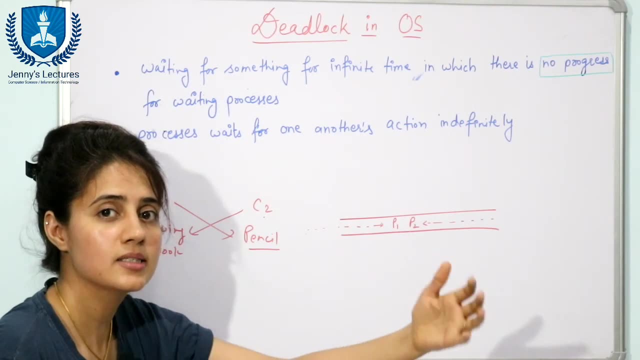 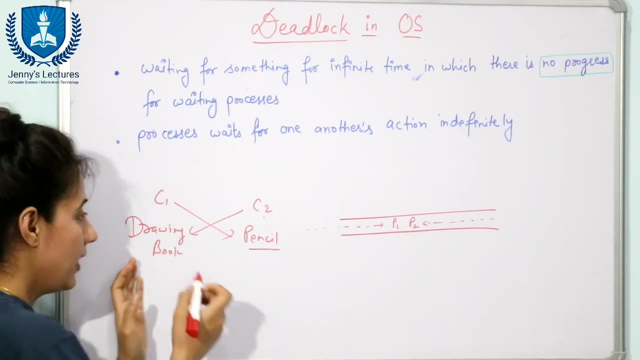 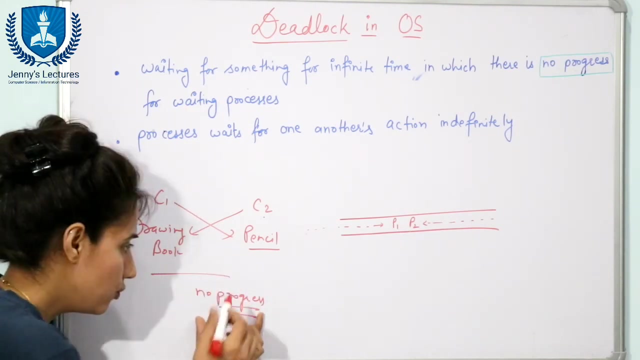 some other waiting process, we cannot say by some other process which are waiting for some, which are waiting for resources, which are held by some another waiting processes. see, this one is also waiting, this one is also waiting, fine, and here no progress case is also there. you can easily analyze that here also no progress case is there. so if no progress is there, 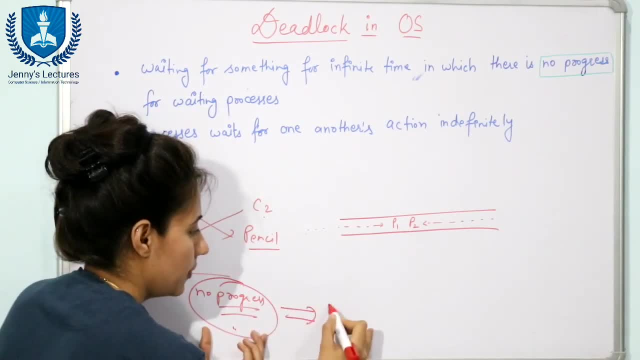 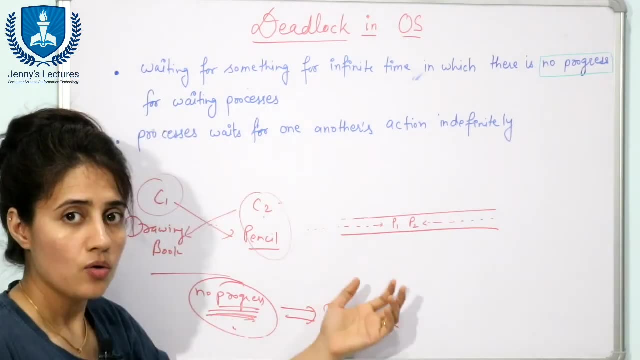 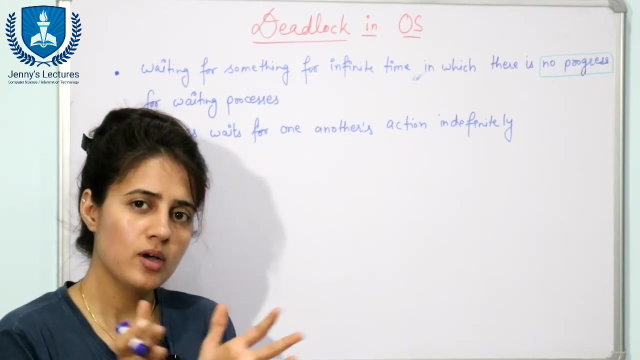 in any situation. then you can say: ultimately there would be deadlock. so this, no progress funda is very important. now come to the point of operating system. see see. basically deadlock comes in the operating system which are in which multiple processes are running. multiple processes are competing for some resources and multiple 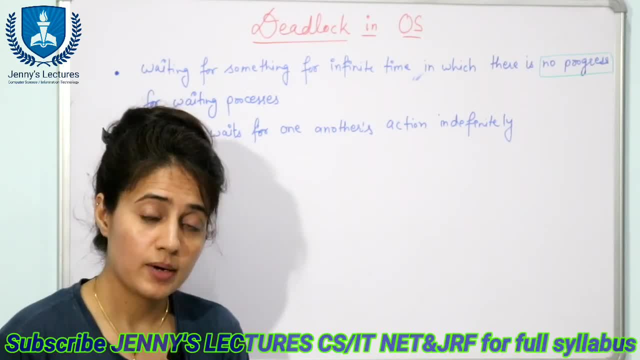 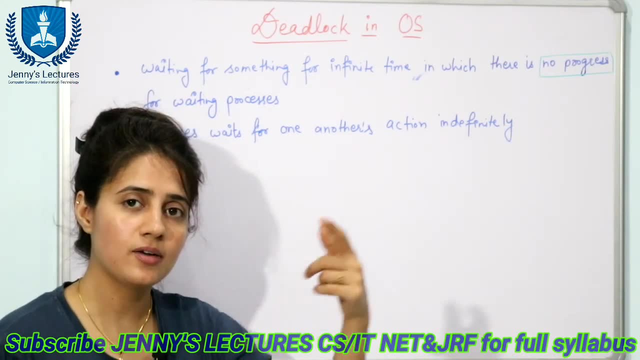 multiple processes will be running. maybe you know, in multi-programming operating systems. see, we have discussed many types of operating system in that video. we have discussed what is multi-programming operating system. so, for example, if you have an operating system and you have many processes going on in a 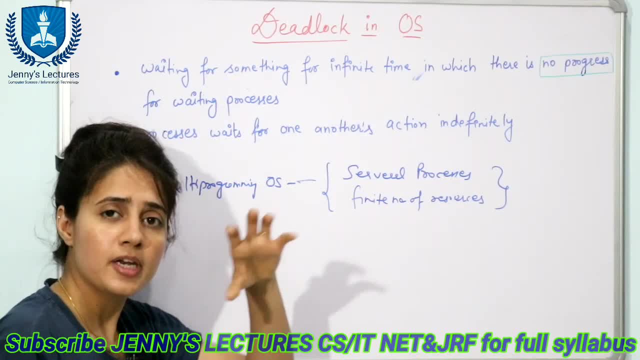 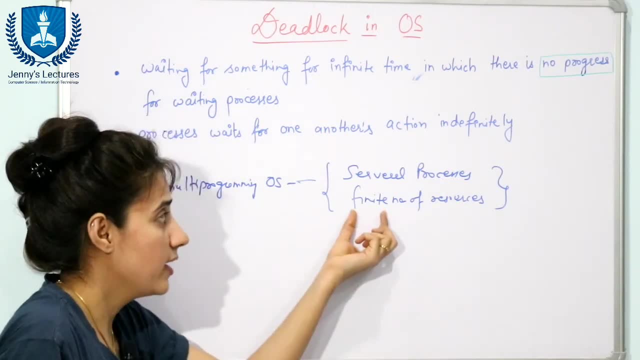 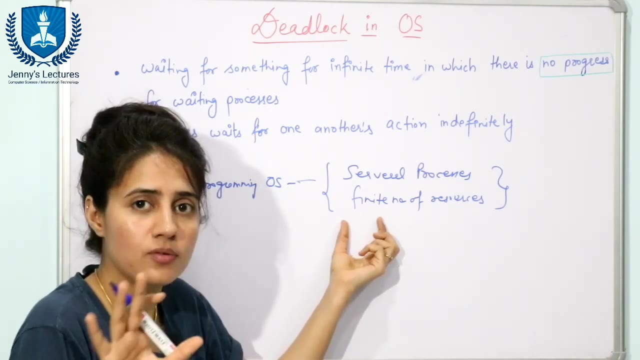 So we can say in multi programming operating system many processes are there, many processes are running and many resources are also there. but resources are finite number of resources. We cannot say: if resources are infinite, then obviously there would not be deadlock and we don't have infinite number of resources. We have some limited number of resources. 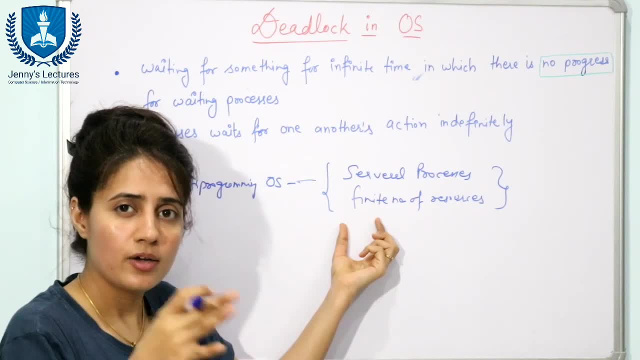 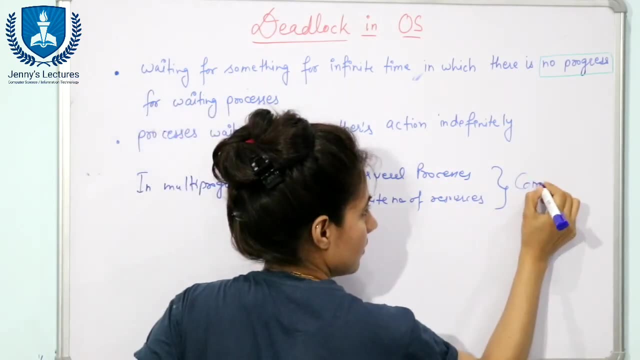 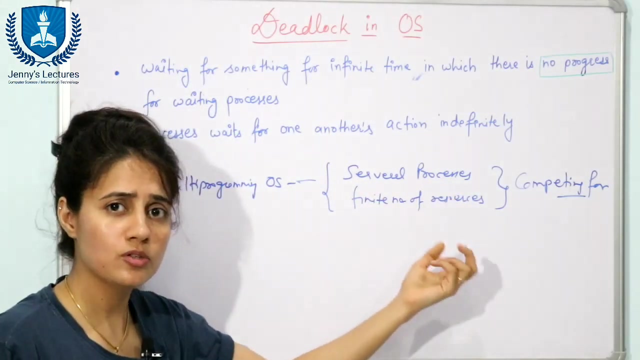 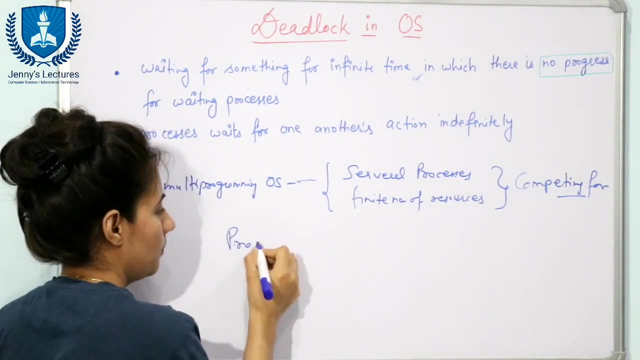 Resources means your CPU, memory, IO devices and all these are resources. Fine, And these processes are competing. Obviously, these processes, multiple processes, are running. then these processes will be competing for these number of resources. Fine, Now, at some time, maybe one process, P1 request a resource. 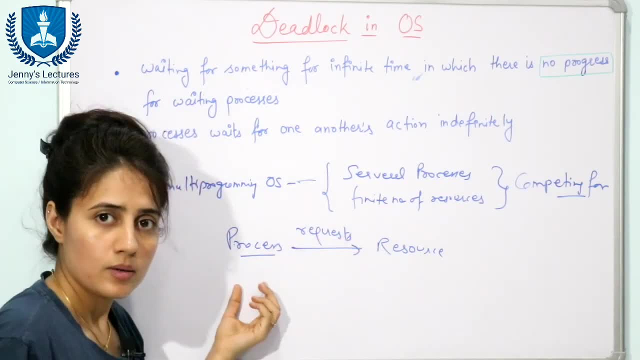 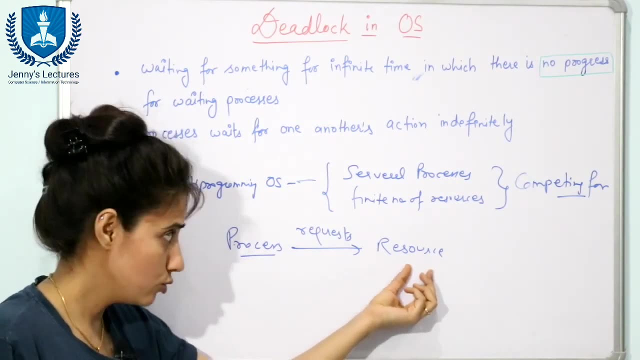 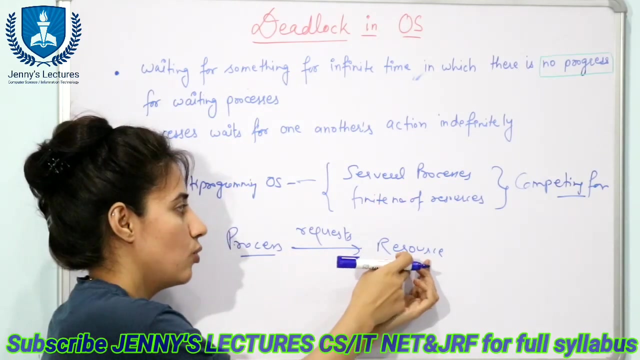 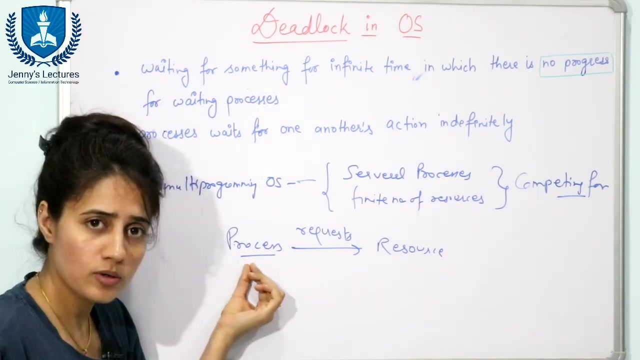 Any process P1 request a resource. If this resource is available, then ultimately this resource will be allocated to this process. But suppose this resource is not available, Maybe some other processes holding this resource or using this resource? Fine, Now, at this point of time, this resource cannot be allocated to this process, then this process will go into waiting state. 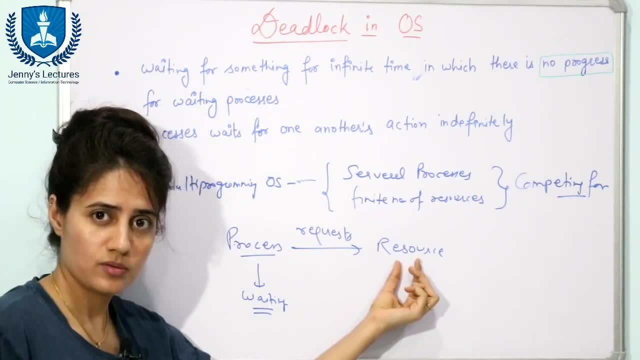 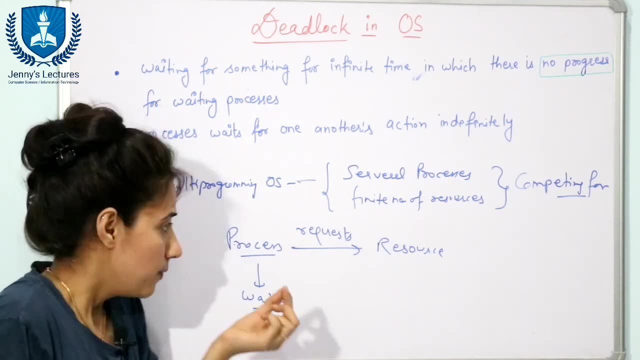 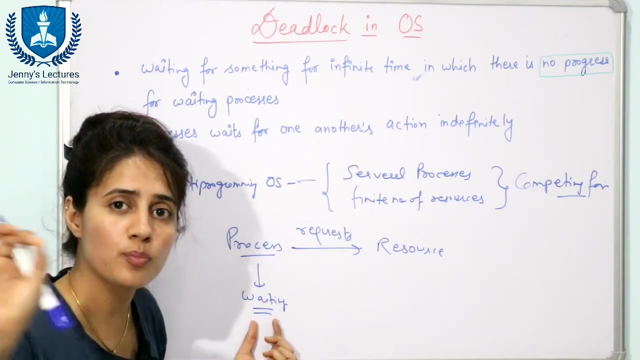 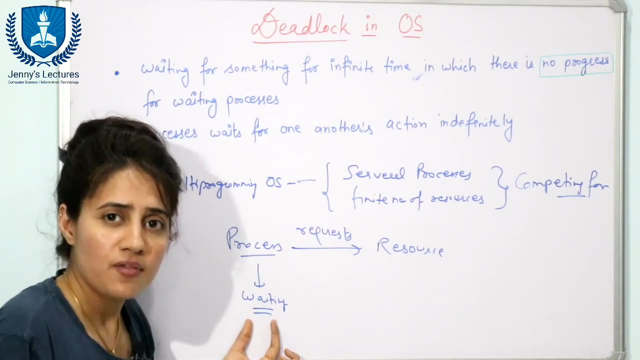 And this will be waiting for this resource. Fine, Maybe some other processes are also waiting for this resource And sometimes this process, this process which is in waiting state or in waiting state, there may be set of processes, more than one process, So sometimes these processes, or you can say this process, never again change its state. 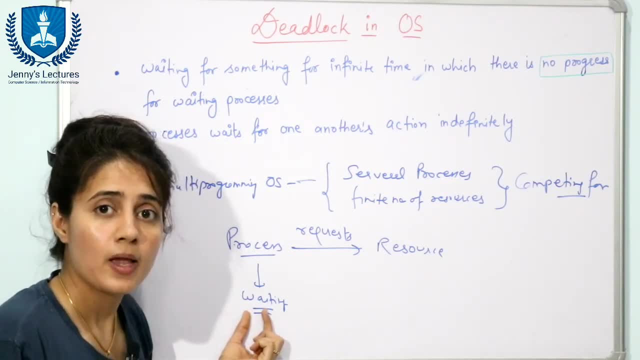 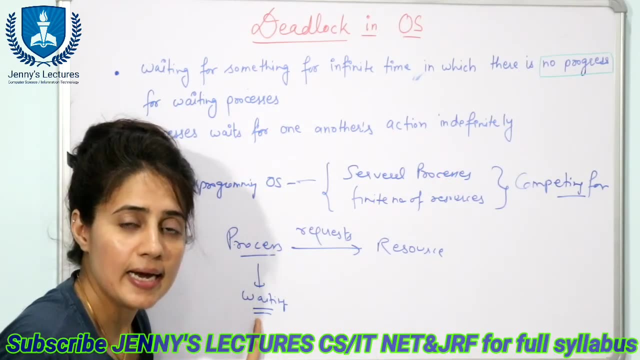 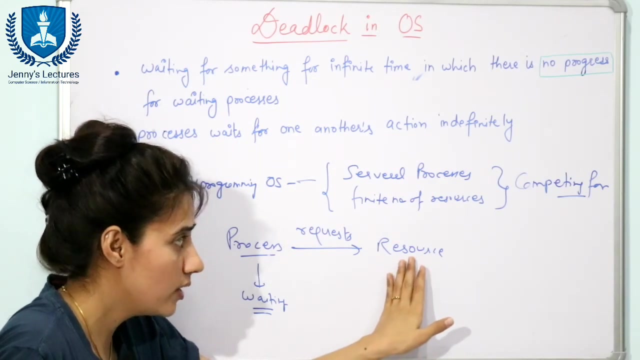 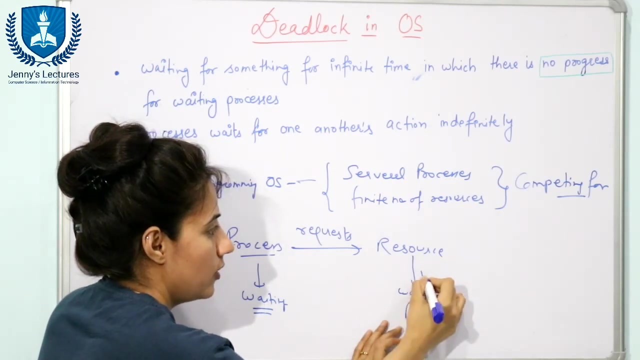 It will always remain in waiting state state. and why so? because this process is waiting for a resource which is already held by another waiting process. another waiting process is there which is holding this resource of that process. suppose p2 is also in waiting state, which is holding this resource. 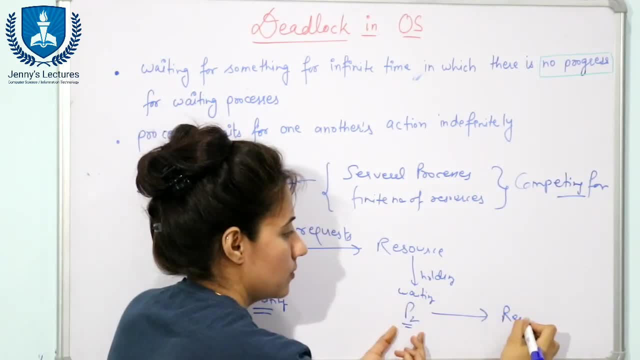 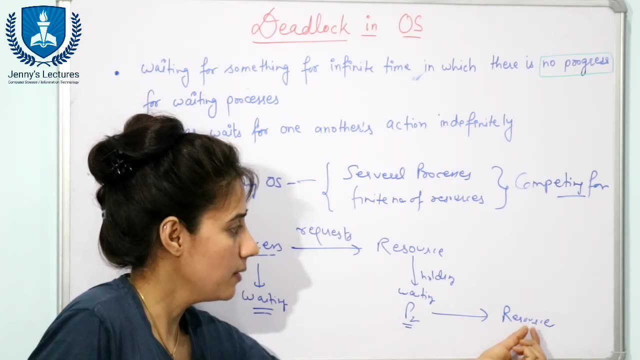 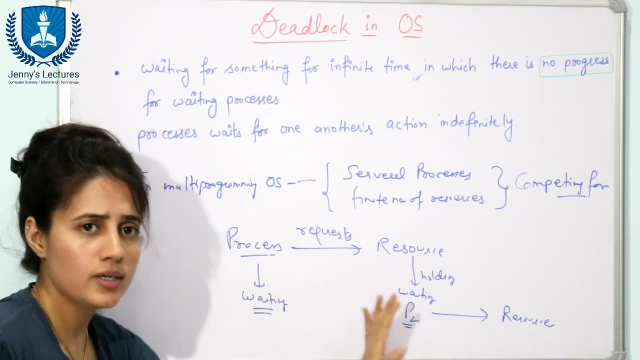 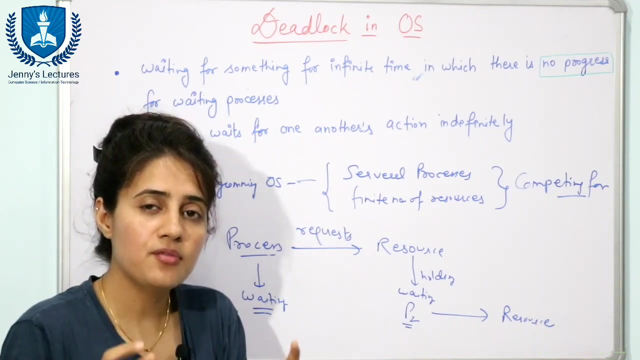 waiting means obviously this would be waiting some another resource, something like this: now this p2 is waiting for a resource again. maybe this resource is again held by a waiting process. so if this kind of scenario is there, then you can say: this is deadlock. now you can say, when a waiting process never again have able to change its state because 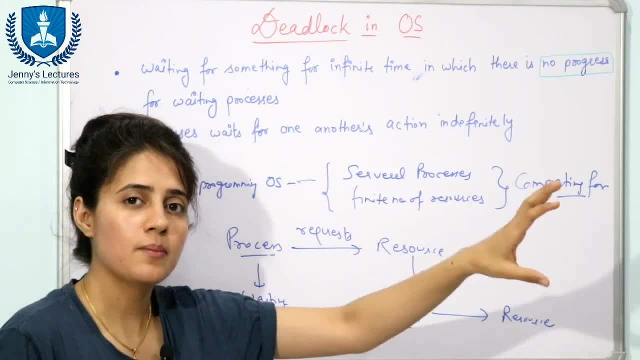 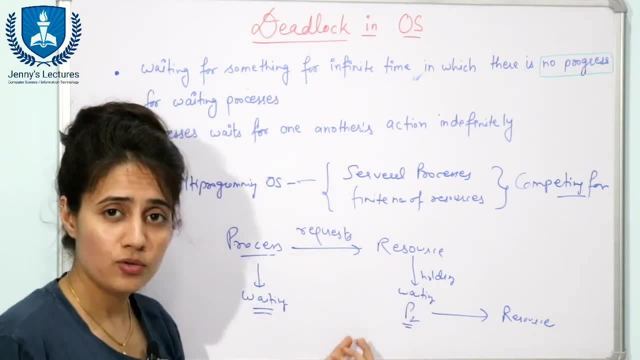 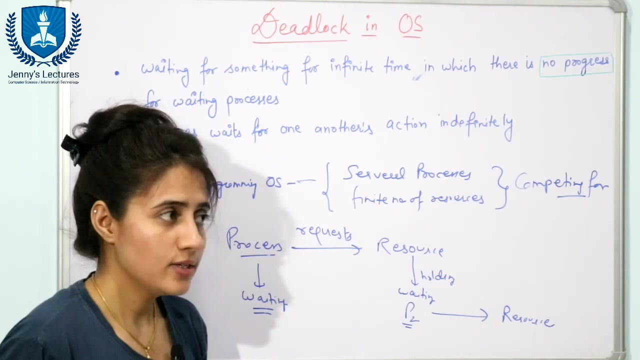 it is waiting for the resources which are held by some other waiting processes, then this situation is known as deadlock. one more point also: you can, you can add in this definition: and there is no progress, then ultimately there would be deadlock. now we'll discuss what are the four necessary conditions. see, i am saying only necessary conditions. i am 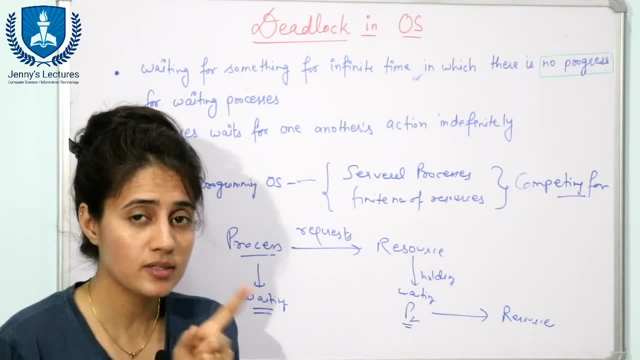 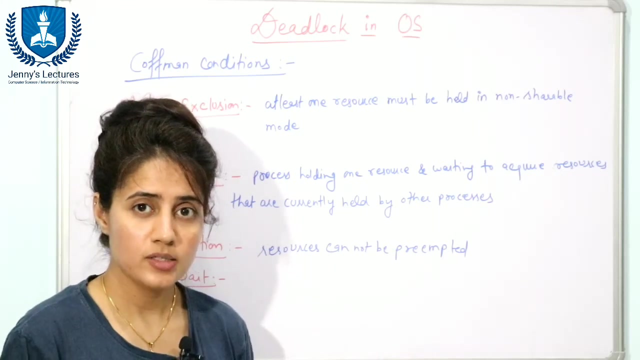 not saying that necessary and sufficient condition condition. you cannot say necessary and sufficient condition, only these are necessary conditions. or you can say kaufman conditions: now four conditions, conditions also. now, these are the four necessary conditions for deadlock. or you can say kaufman conditions for deadlock: one is mutual exclusion. second, one is hold and wait. next is no preemption. 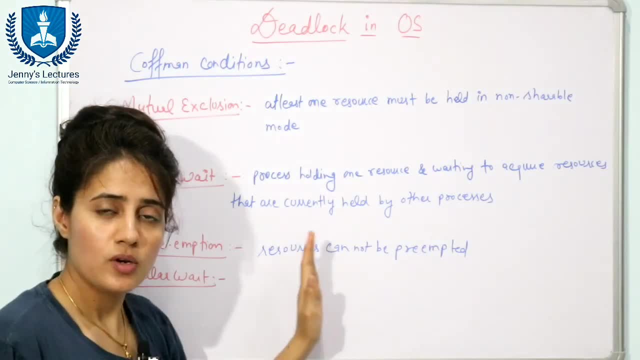 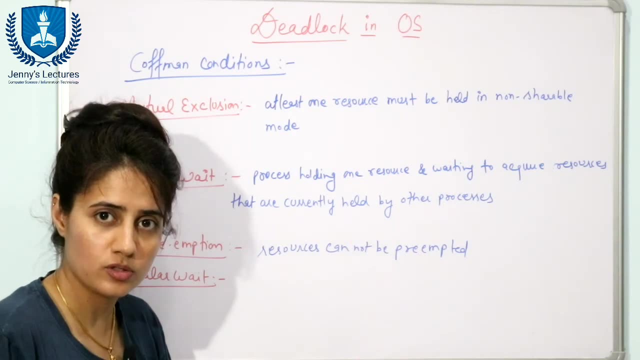 and next one is circular weight. so deadlock situation will arise if all the four conditions held in the system simultaneously at the same time, all the four conditions, not only one, only two or only three. no, on the all the four conditions are there, then deadlock would be there in the system. 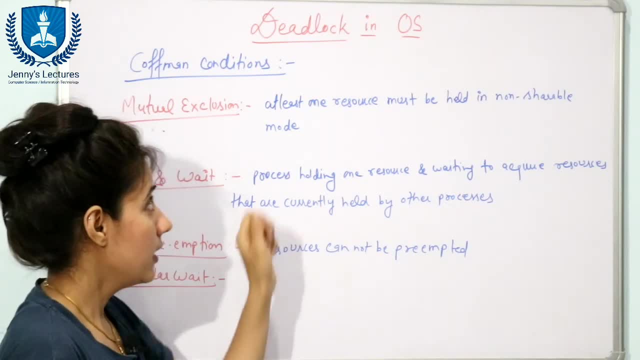 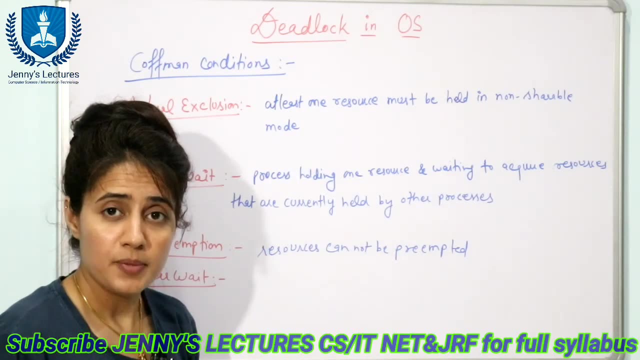 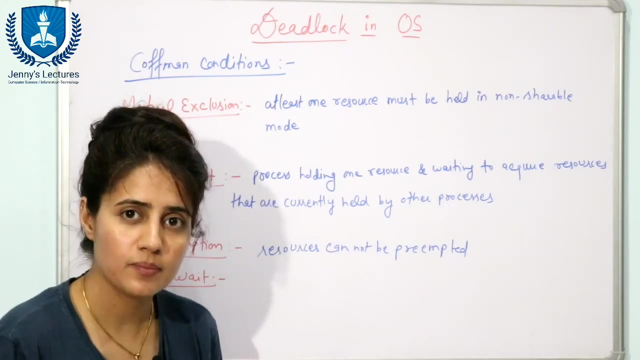 now, what is this? mutual exclusion in this case we can say at least one resource must be. must be held in. a non-shareable mode means we cannot on only one process. non-shareable mode means only one process can use a resource at one time. no two process can share the resource. any other process wants that resource, then that. 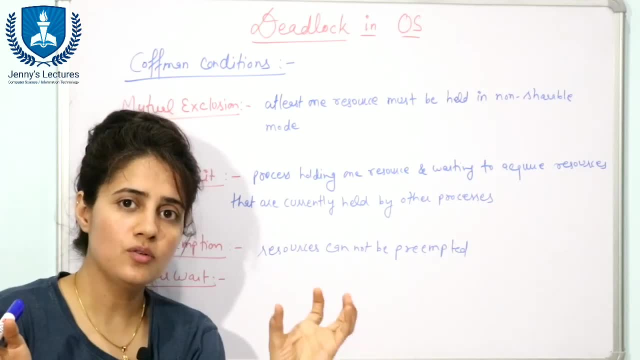 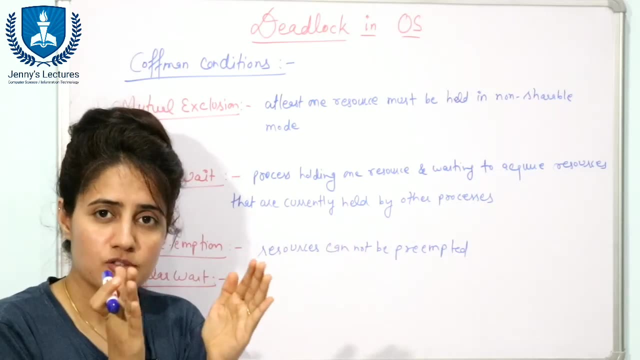 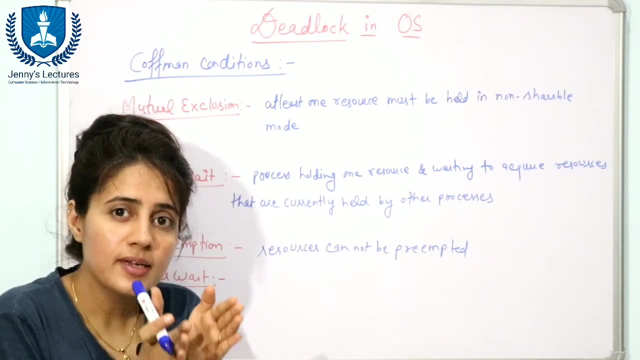 second process has to wait until the completion of the first process. this is first condition: mutual exclusion. we have taken the example of this: that street, narrow street, so that is non-shareable. why you can say non-shareable? because only one person can pass through that street, and what? at one. 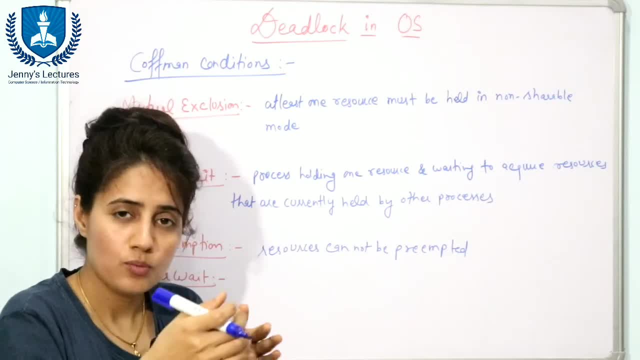 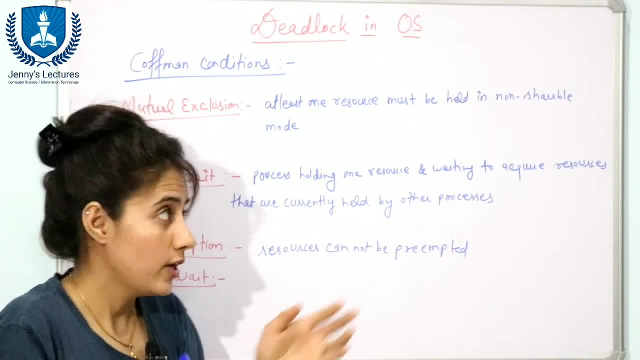 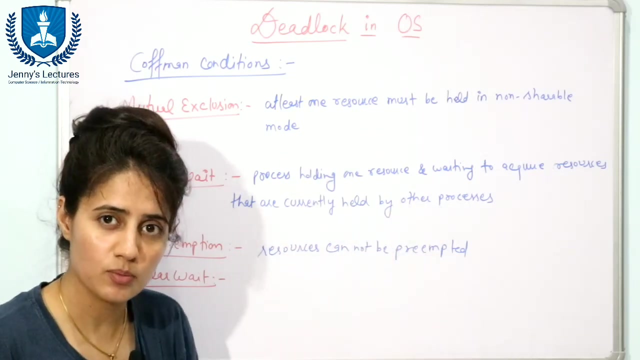 amount of, at particular amount of time, if both the person, if two person can pass, then that is, you can say uh, shareable, and at that time there would not be deadlock. so that is why this condition should must be hold in the system. at least one resource would be there must be held in non-shareable mode. 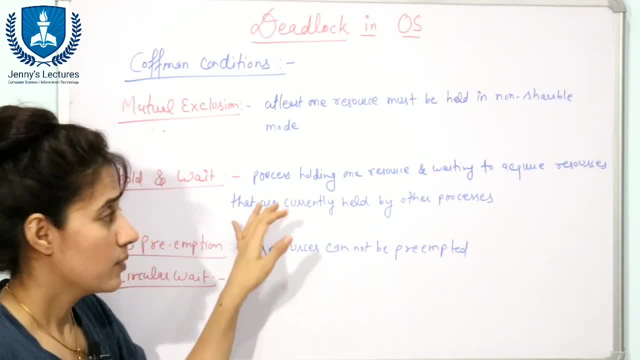 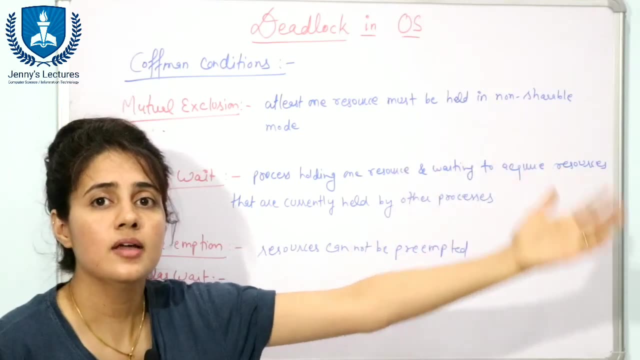 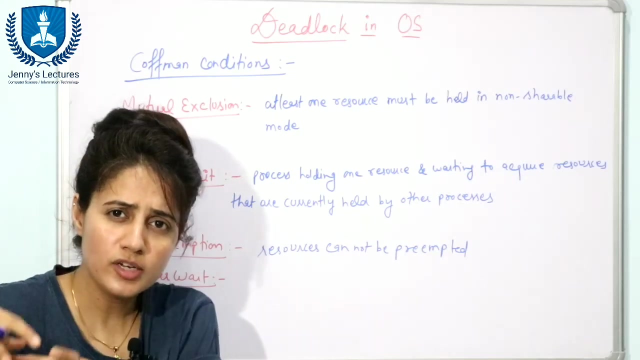 now next. next one is hold and wait. it means processes must be holding some resource and waiting to acquire some other resources that are currently held by some other processes. it should not be a case that if you are holding some resource, you cannot wait for or you cannot. 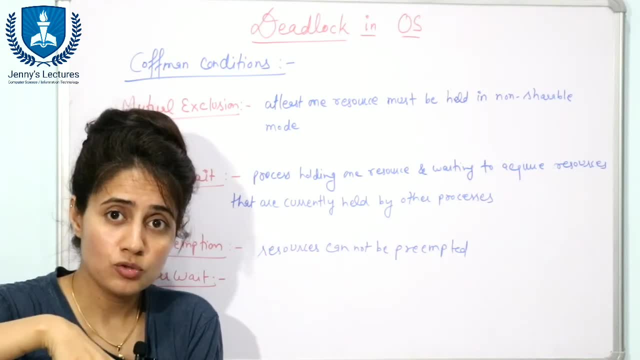 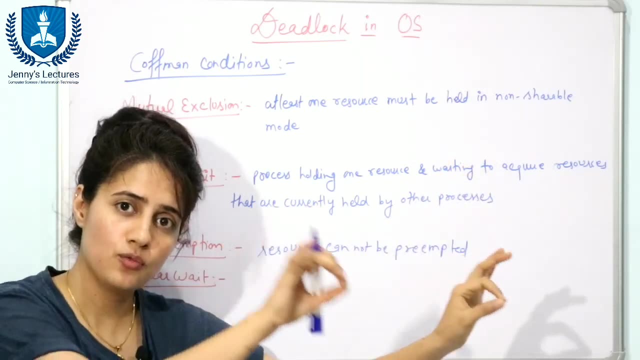 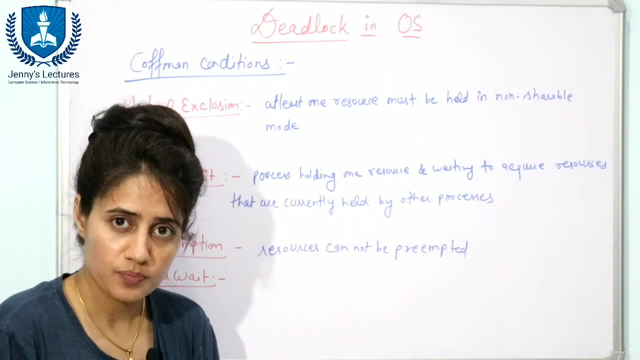 request for another resources. no, you are holding maybe resources r1, r2 and you are waiting for resource r3 and r4. that should be a case hold as wait. you can hold some resources also process, can hold some resource also and can wait or request for another resources also. third is no preemption. i have discussed this preemption. 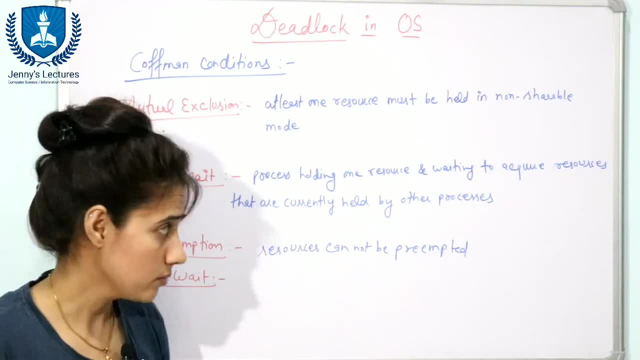 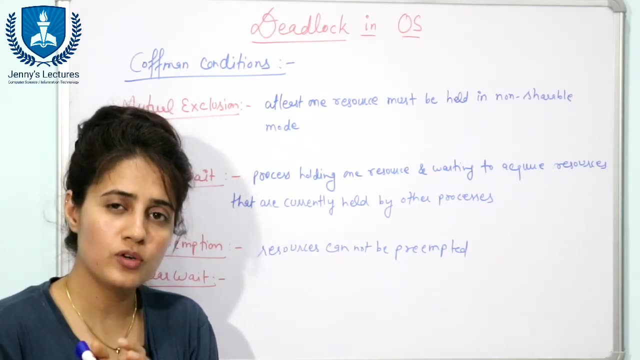 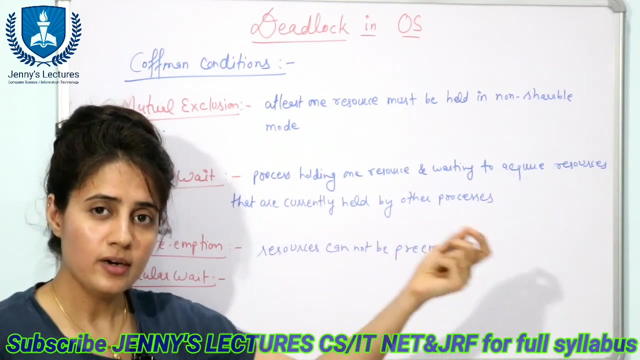 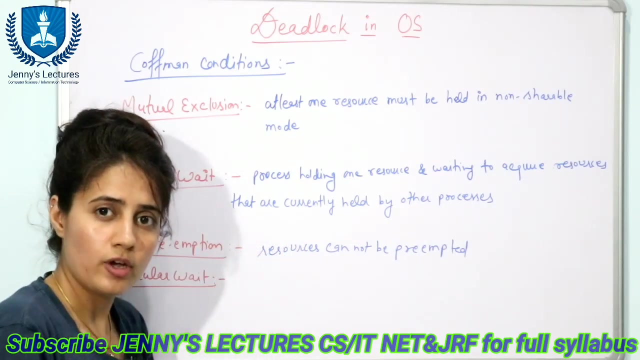 many times means forcefully, you can remove something. so no preemption means resources cannot be preempted. if one process is holding some resource, we cannot forcefully take that resource from that process. no preemption would be there. see, in case of that drawing book, end pen maybe, uh, forcefully from one child we, we took the drawing book and give it to the second. 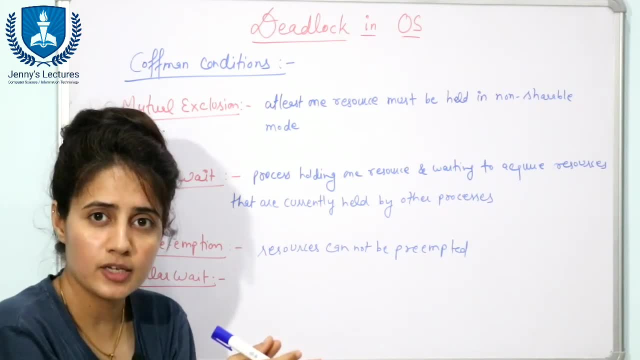 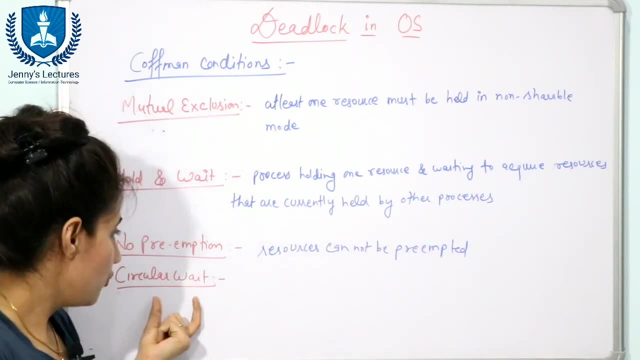 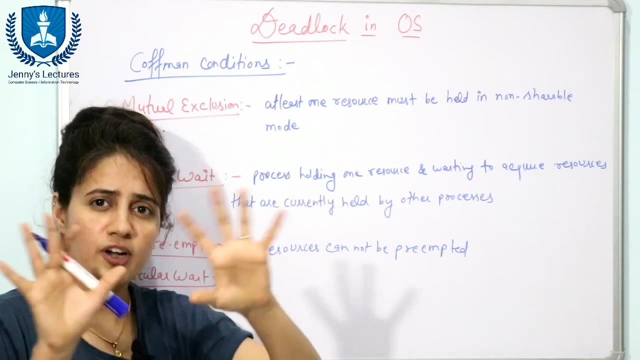 children, then obviously there would not be deadlock. but that should not be a case. you cannot forcefully take any resource from a process. no preemption case would be there. and last one is circular weight. circular weight means they are waiting in circularly, like suppose we have processes from five processes are there p1, p2, p3, p4, p5? 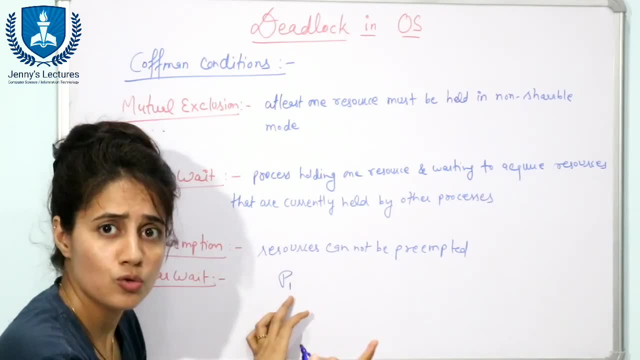 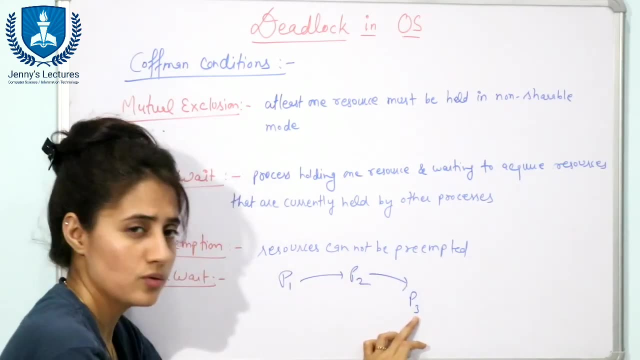 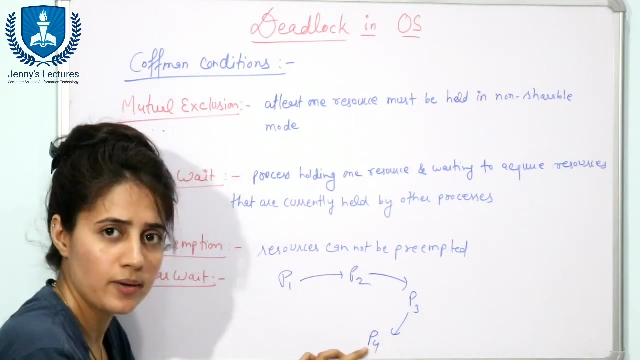 and p1 is waiting. p1 is waiting for a resource and that resource is held by process p2. p2 is waiting for a resource. that process is held by resource p3, by process p3. p3 is waiting for a resource that is held by process p4 and p4 is waiting for a resource that is held by. 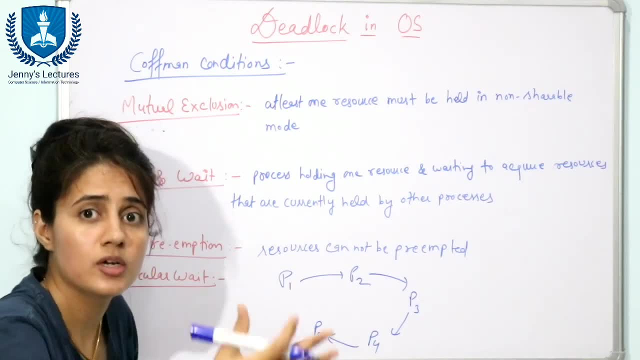 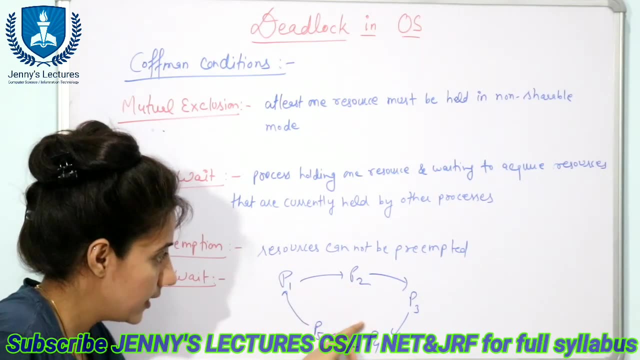 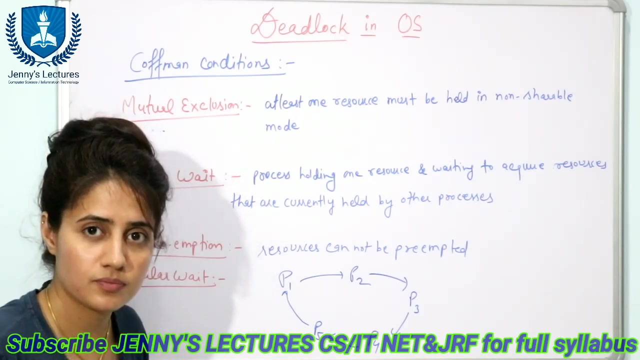 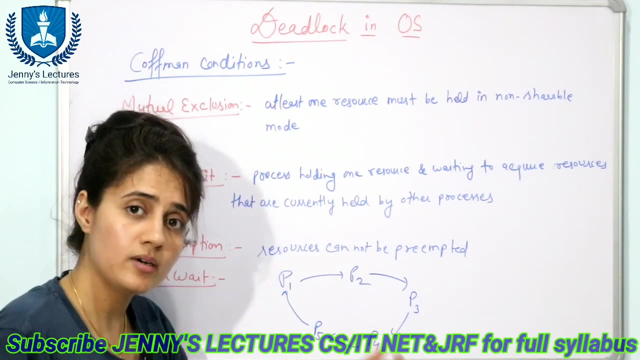 p5. and finally, p5 is waiting for a resource, and that resource is held by process p1. this is a circular weight condition, so this would also be there, otherwise deadlock would not be there. fine, so all these four conditions must be held simultaneously in a system, then a deadlock. 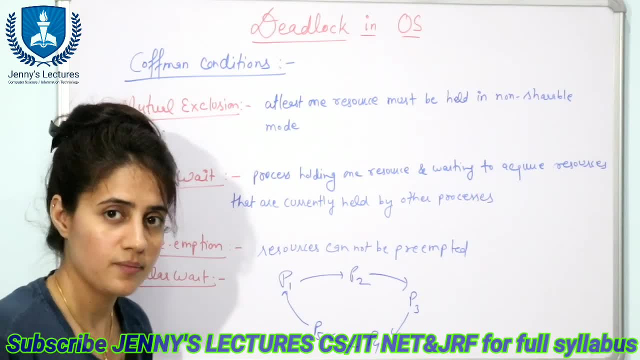 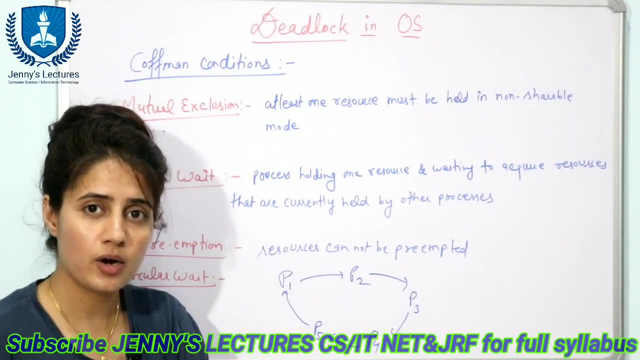 situation arise, fine. so in next video we'll discuss how to pre have to handle the deadlock, how to prevent, how to avoid, how to detect the deadlock, how to recover the deadlock bankers algorithm and all fine. so till then, bye, bye, take care.